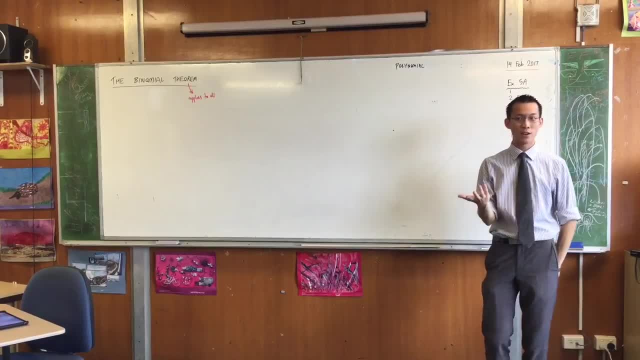 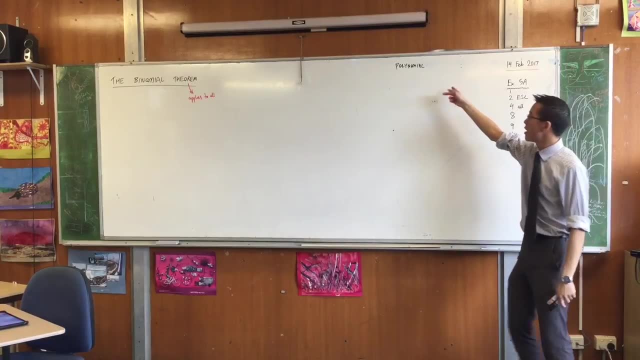 Poly means many, So, for example, polygon, many angled Polystyrene, many molecules of the same that are all strung together. That's the way plastics are: Polynomial: many, and this is a bit tricky, but essentially, for our intents and purposes, it means terms. 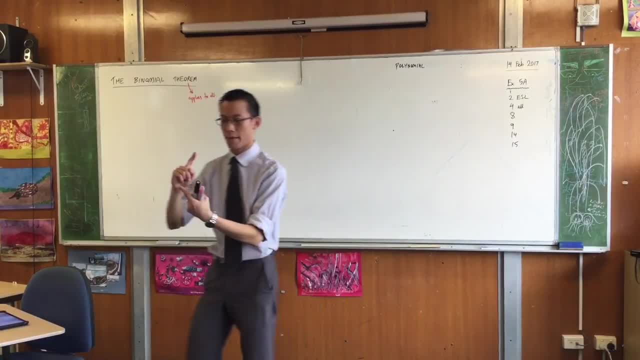 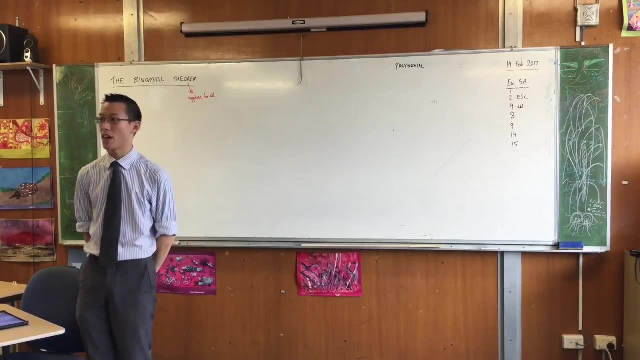 Do you remember? right at the beginning of the year, we were talking about algebra. We said there are expressions, equations, coefficients, Terms are just, like you know, x cubed 5x to the 7. Those are terms and a polynomial has lots of them. 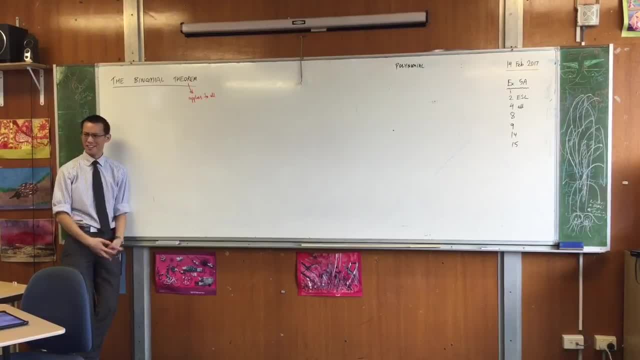 How many does a binomial have? Two, Only two. You're like: what Bit of a step backwards, isn't it? We worked with polynomials before. Well, believe me, we'll get there. Binomials have plenty of things up their sleeves. 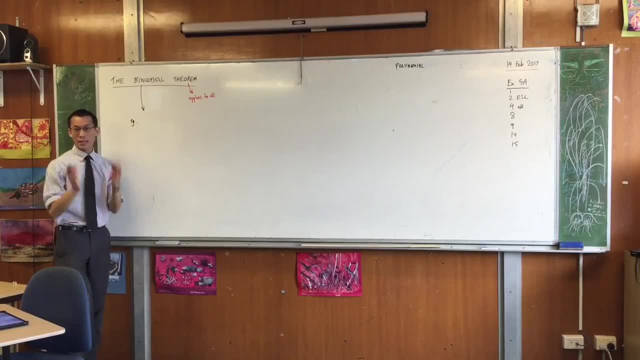 So, as an example right, A typical polynomial would be something like sorry binomial. rather would be something like x plus 1.. This is a binomial. It's got two terms. I can see that they're clearly different. 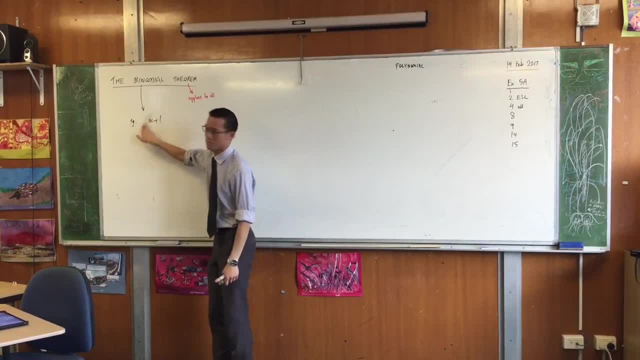 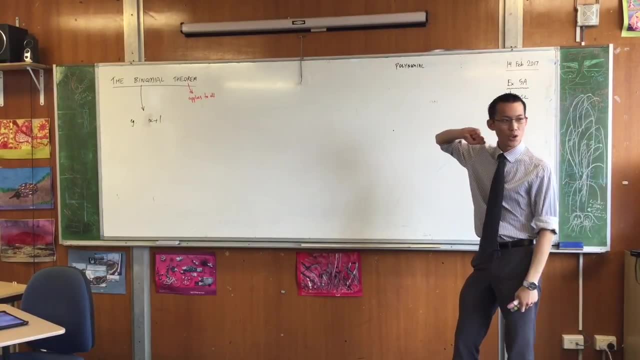 There's no way to collect them together, Unless you know what x is, and then you're not collecting anymore, You're evaluating. So this is a binomial, okay. The binomial theorem has to do with what happens when you take this thing and you raise it to a power. okay. 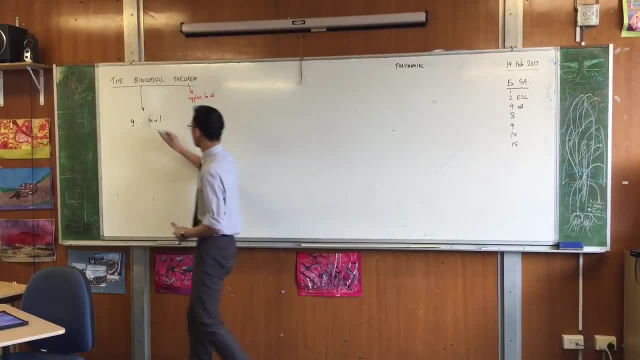 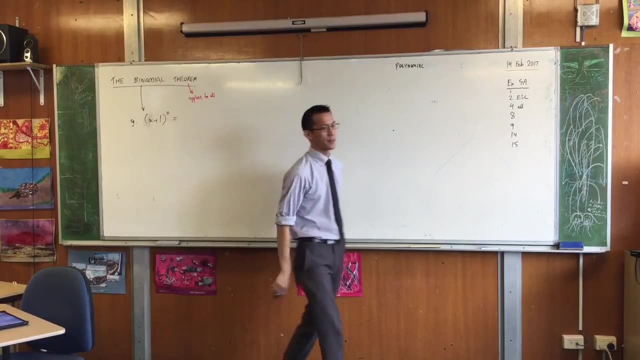 Particularly integer powers, So let's begin with the first one. The first power that we're going to think of seems a bit trivial, but it's 0, okay, Mathematicians like to start counting from 0 a lot of the time, and this is one of them. 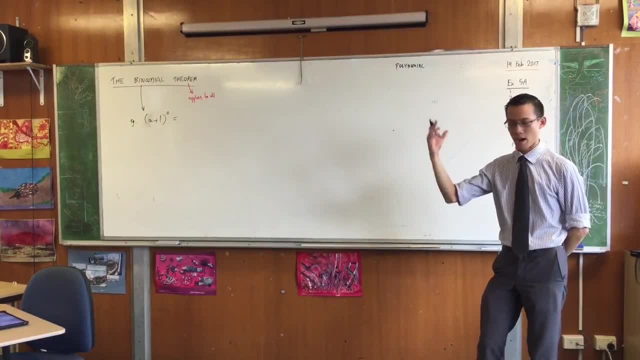 Now, when you raise anything to the power of 0,, 1, to the power of 0,, 15 to the power of 0, negative pi to the power of 0, what do you get 1.. You get 1.. 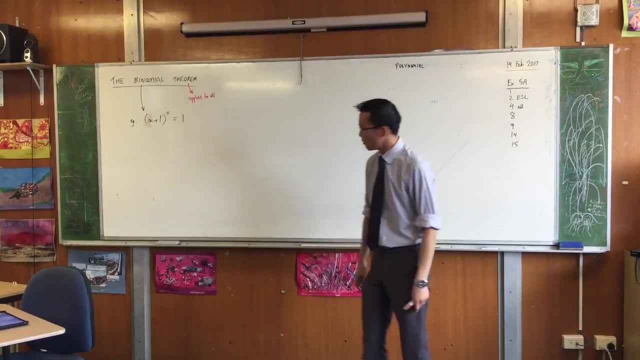 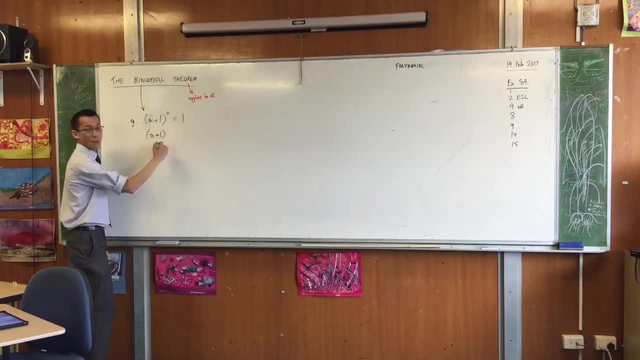 Every single time, no exceptions, okay. So not much interesting is happening at the moment. Let's have a look at what happens when we increase the powers. If I go to the next one and remember, I'm thinking about integers, so the next one is just 1.. 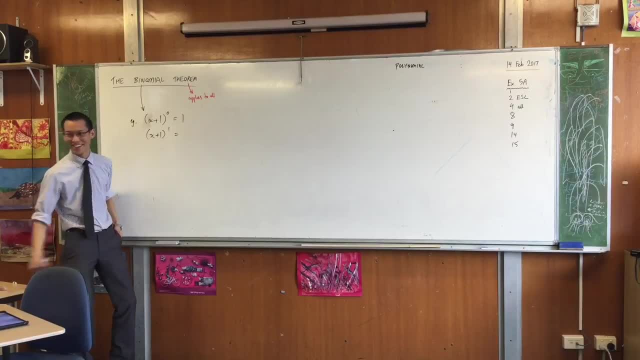 You're like, wow, this really is 011 Maths, isn't it Okay? x plus 1,. again, not much interesting is happening. Nothing is happening just yet. Here's where it sort of begins to take off, and we've looked at some of these back under our previous topic, right? 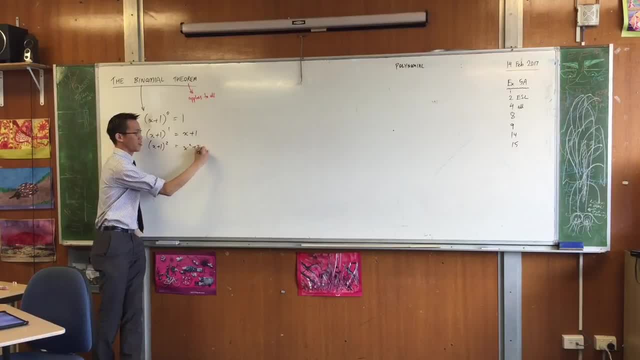 We know by definition. we know this pretty well. This is just a perfect square, And last time we were looking at cubic identities, so we should know this one reasonably well. Can anyone recite it Now? just pause for a second. If you cannot recite it, that is fine. 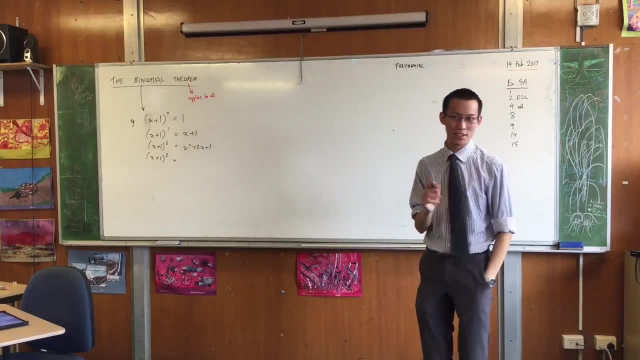 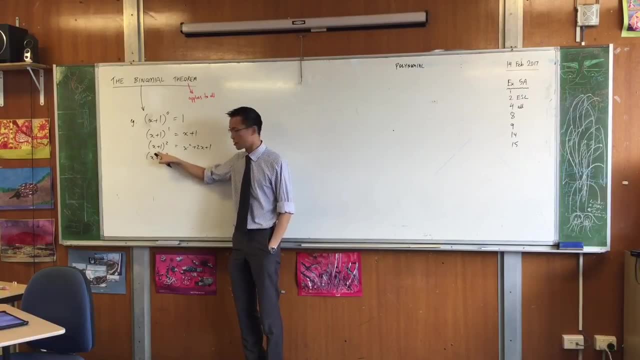 By the end of this topic, you will be able to. We can actually do a little bit of trickery here to take advantage of the work we've already done. Do you agree that this is just this times, this, Do you agree? So I'm just going to do my pairing up of all my terms. 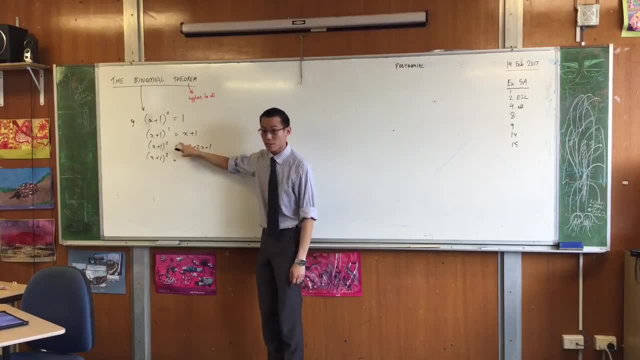 I'm going to take everything in here and I'm going to multiply it by x. Then I'm going to take everything here and I'm going to multiply it by 1. And then I'll just take the sum. That's all I need to do. 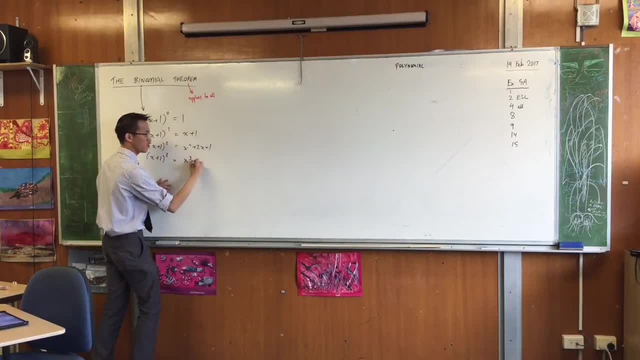 So we'll multiply everything by x first. That'll give me x cubed plus 2x squared plus x. So there's x times that, And then I have to add on plus 1 of this. Now, for reasons that will become clearer in a second, I'm going to put this on the next line. 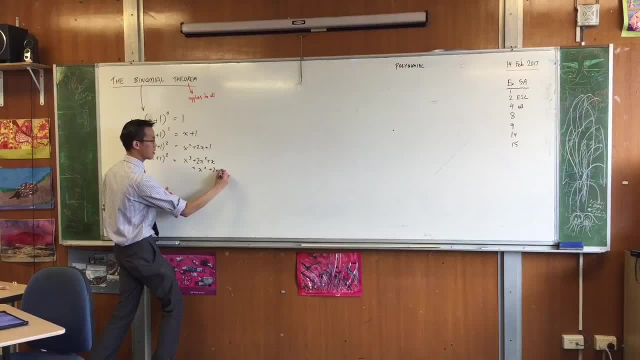 I'm going to put the x squared here and the 2x here and the 1 there. Can someone tell me why I interleaved it this way? I'm trying to identify the like terms. Do you see those? Yeah, they're cold. I remember now. 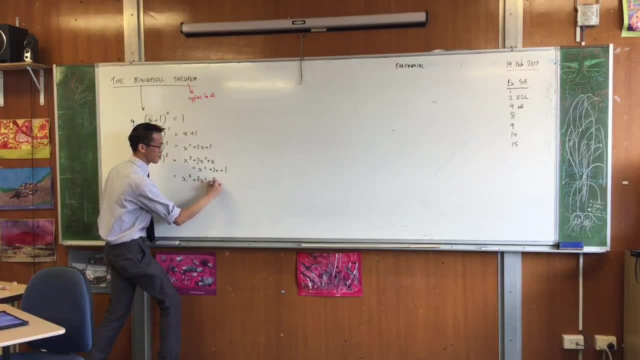 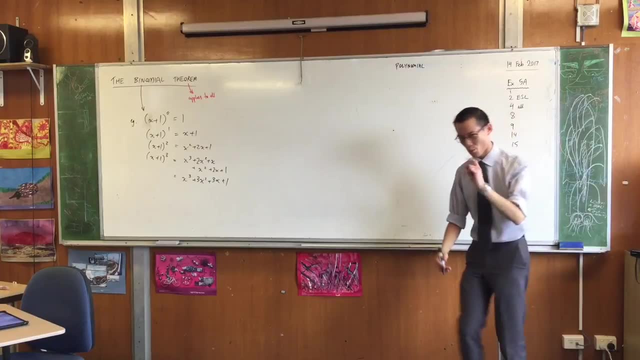 x cubed. you can see there are 3x squared, there's 3x's and then there's a 1 here. Now you're like: alright, fine, we got there. I want to do this one more time. 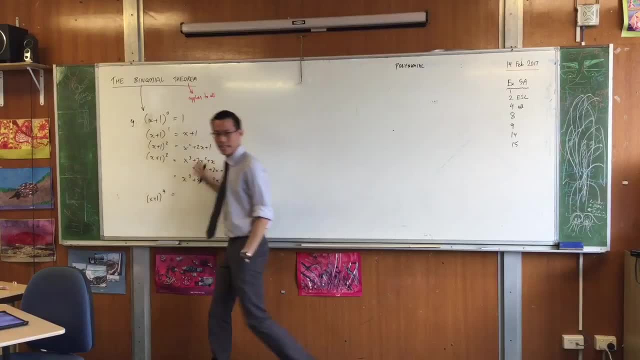 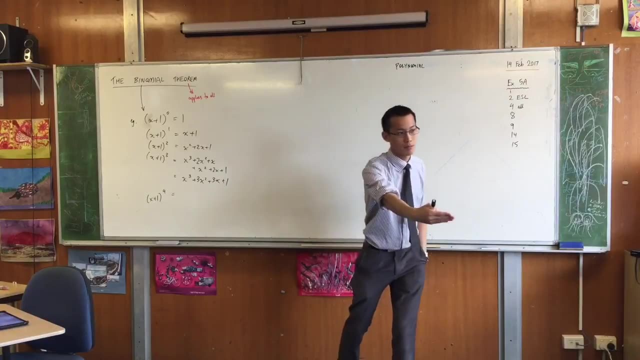 One more time, And because of this technique that I've just developed, which is that if I know what this one is, the previous one, I just do the same thing again: I'll multiply every term by x, then I'll multiply every term by 1, and I'll just add those up. 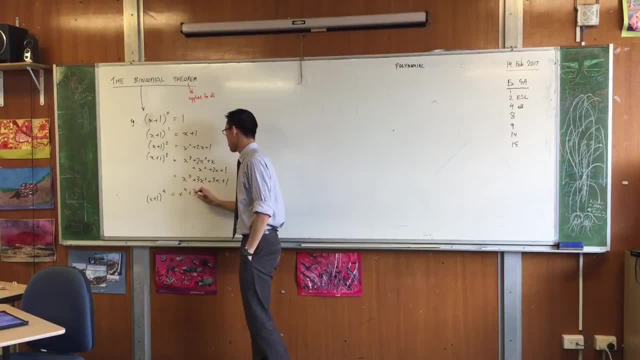 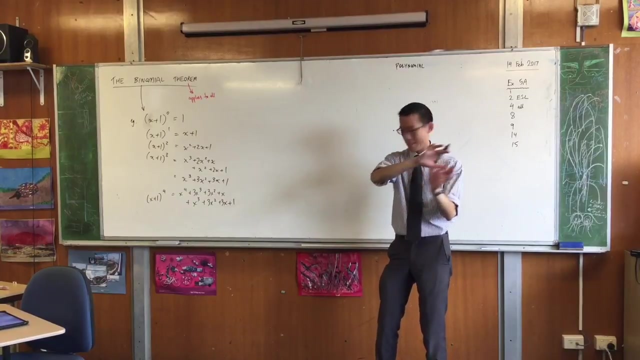 That's not difficult, So let's have a go. You get x to the 4, 3x cubed, 3x squared, Then you get. You see the way I did it, The structure there. it's not just like a stream of unrelated symbols. 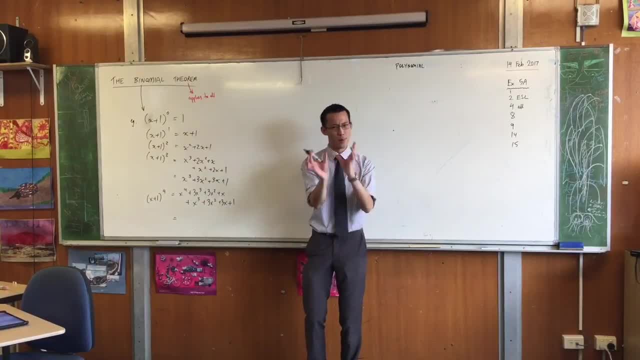 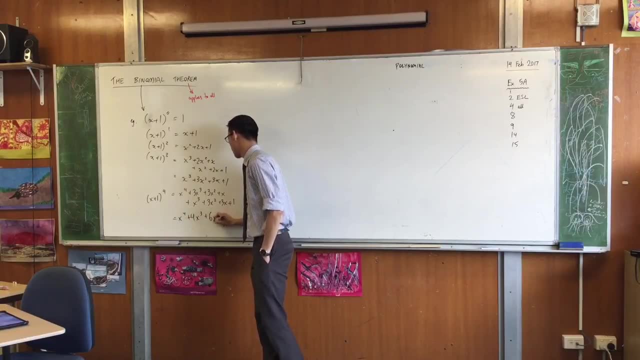 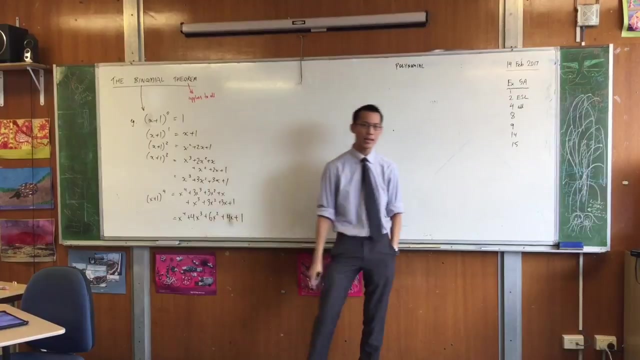 You see, I told you we'd get to the polynomials, And now I'm going to line up all of the like terms. So I've got a single one of these, Four of these And one of those. Okay, So I could make you do the next one, but I think that's enough to make the point. 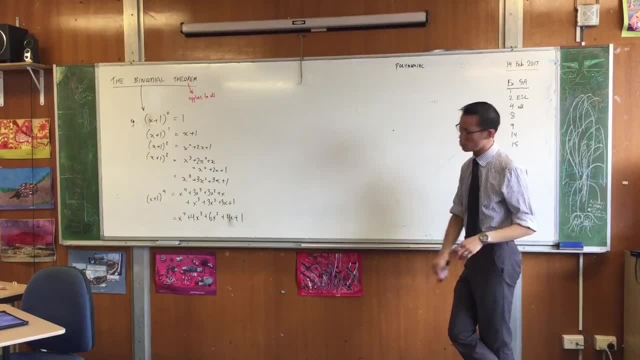 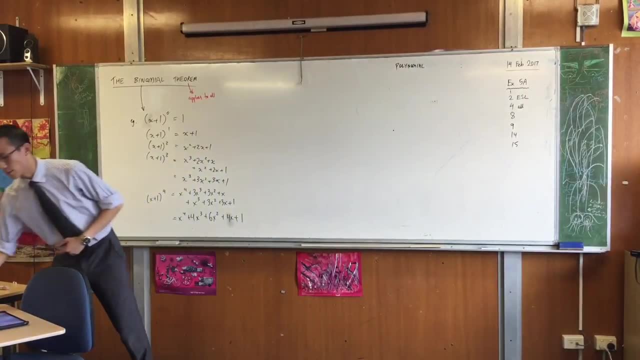 What are we looking at here? I particularly want you to pay attention- and I pointed this out back when we were looking at cubic identities- When you look at the coefficients. in fact, if you've got another colour there, let's highlight them. 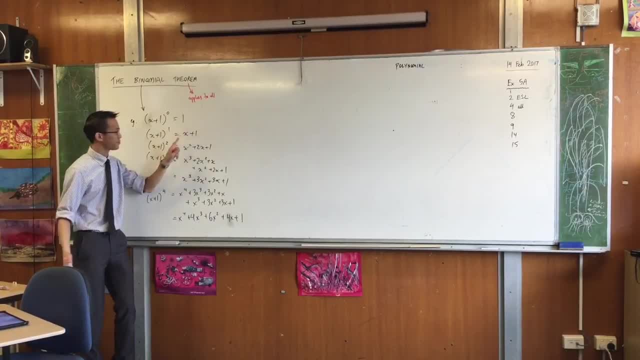 Here there's just a 1. Nothing much happened, But already here we have something interesting. There are two coefficients here. I haven't written one of them, though, because when you've got a single x, you don't need to say a single x. 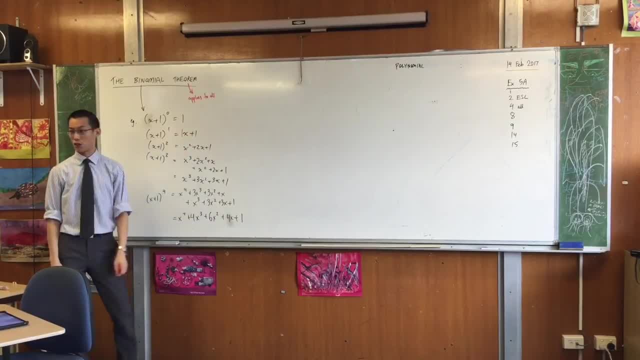 You just say x, But there is indeed a coefficient of 1 hiding there. In the same way, there's always going to be a coefficient of 1, in fact Like that, And you can see. there's this pattern, There's symmetry, you notice. 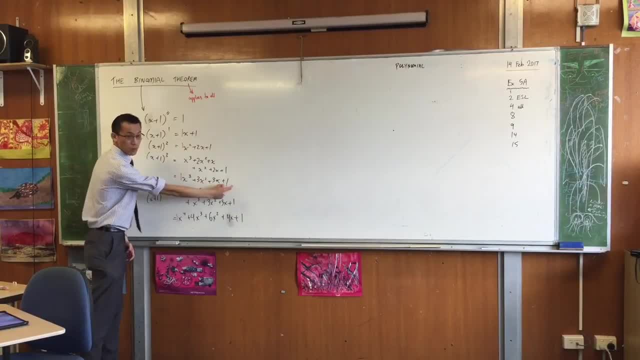 1, 2, 1.. 1,, 3,, 3,, 1.. And then the last one we did was 1, 4,, 6,, 4, 1.. 1,, 3,, 3,, 1.. And then the last one we did was 1, 4,, 6,, 4,, 1.. 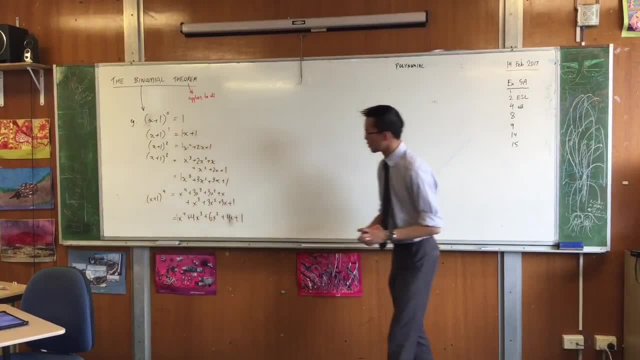 And then the last one we did was 1, 4, 6, 4, 1.. Right, So that's weird. I'm going to point out something else that's weird. I asked you to look at the coefficients. 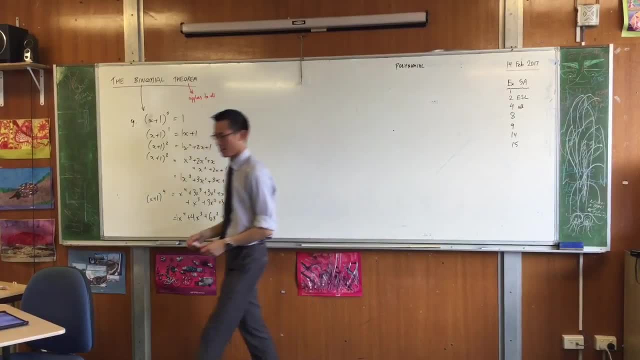 Now I want you to look at each one of these lines And I want you to add the coefficients each time for each individual line. Humanly, what's the sum of the coefficients over here? Sum of the coefficients. Sum of the coefficients. 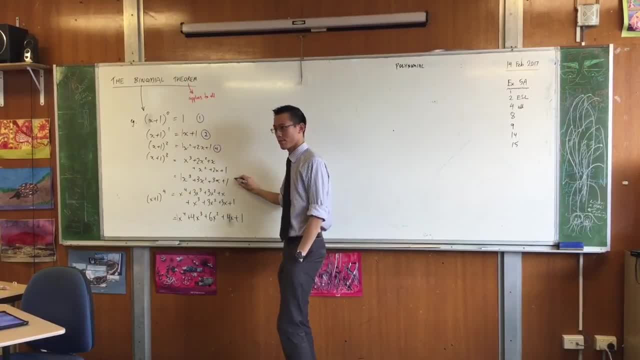 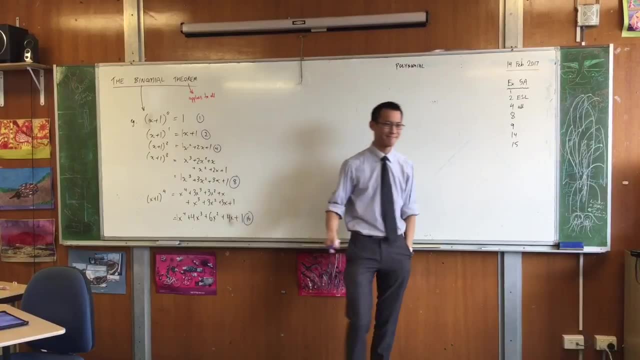 That's 4.. Sum of the coefficients 7,, 8,, 9,, 10,, 11,, 12,, 13,, 14,, 15,, 16,, 17, 18.. Huh, So there's something going on here. 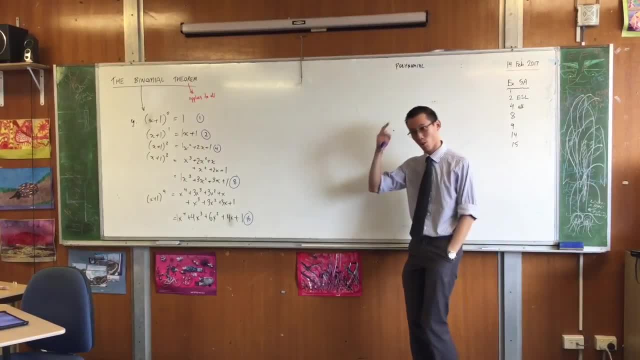 There's something weird going on here And hopefully some cogs are turning And you're recognizing. actually these numbers are not just sort of coincidentally coming up. The next one's going to be 1, 5, 10, 10, 5, 1.. 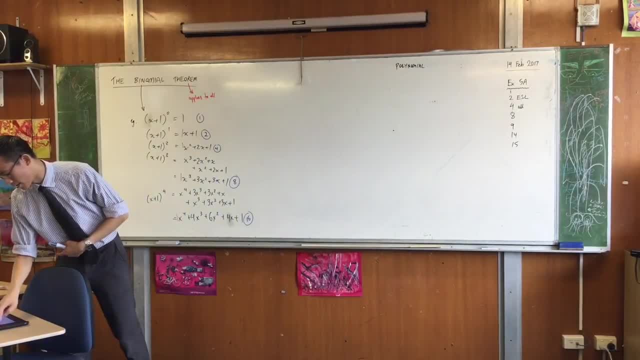 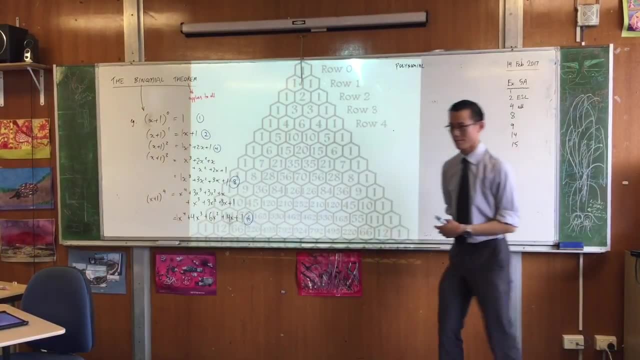 Because these coefficients you may recognize as The numbers that appear in this guy. So this, of course, is Pascal's triangle And you can see up in our top rows there- and yes, there is a row 0, you can see the coefficients that we have just generated. 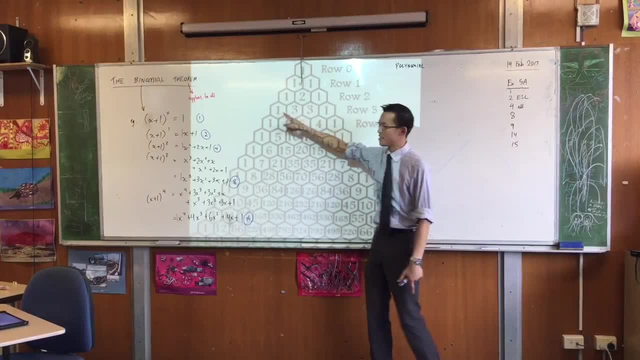 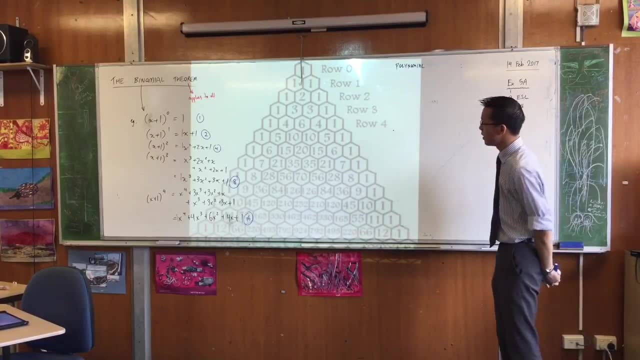 There's the x squared plus 2x plus 1.. There's the x cubed plus 3x squared plus 3x plus 1, and so on. Now you're going to make your own Pascal's triangle in a minute. 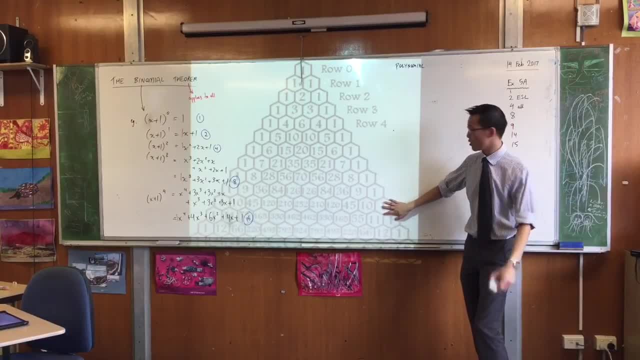 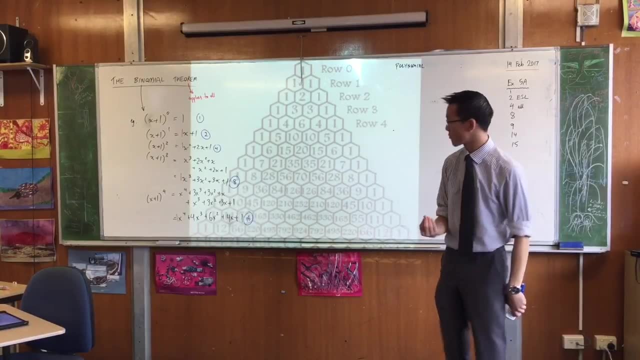 But I just want to point out this is weird, Right? You may have just noticed that every row of Pascal's triangle adds up to 1,, 2,, 4,, 8, 16.. They're not just multiples of 2.. 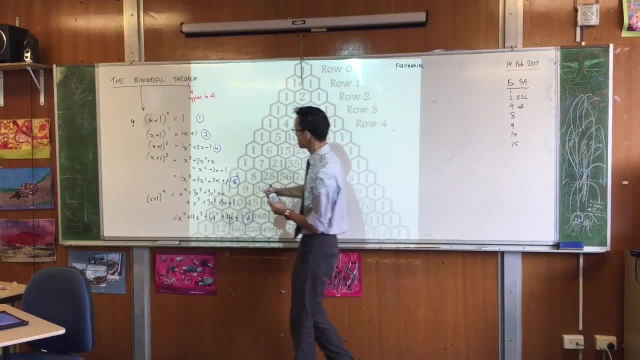 They're powers of 2.. Do you notice that? Because this, This is 2 to the 0.. 0, 0.. This is 2 to the 1.. This is 2 squared And you get the idea. 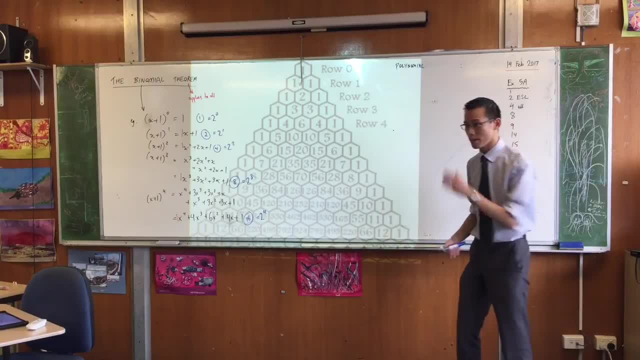 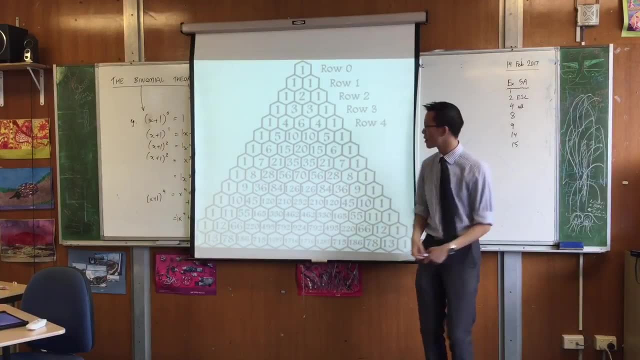 That's weird. That's weird. Right, There's more weirdness happening in Pascal's triangle. I'm going to need a bit of space. I want you to look carefully at the numbers And I want you to think of. Just have a look. 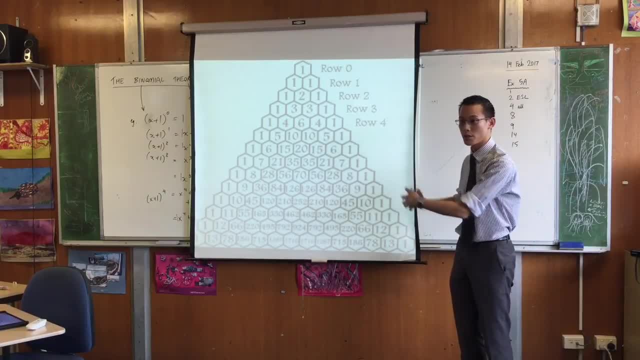 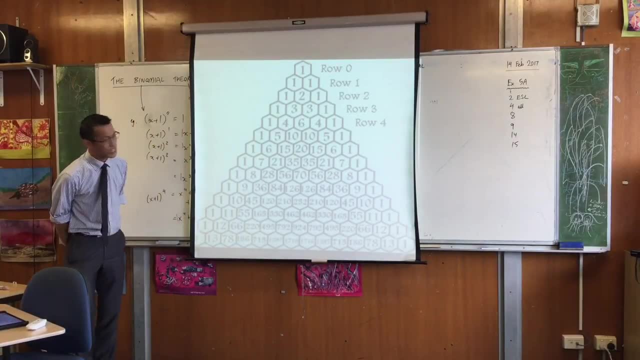 Where are the even numbers in this? Don't say anything. There's lots of them, obviously. I just want you to look at where all the even numbers are. Can you see where they are? It's a bit hard when you're just trying to look at it and just see it. 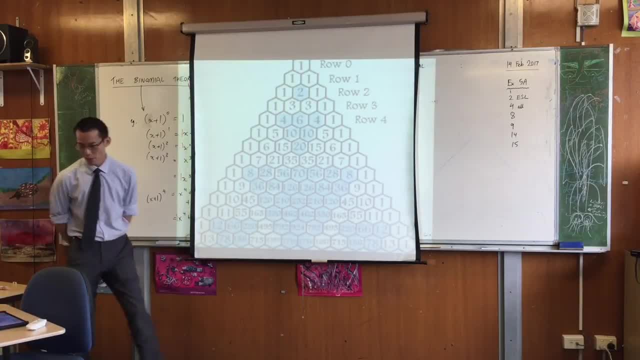 so I'll sort of give you a bit of a hand. Here are all the even numbers. Let me turn off the laptop to be clear for you, Because it's a bit dim. Can you see them in blue? I know it's a bit dim. 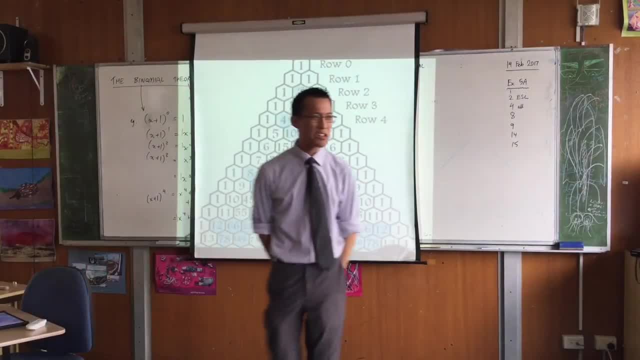 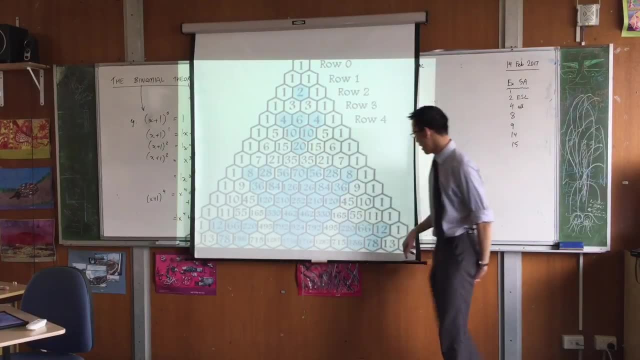 Can you see them? Do you notice? there's kind of a weird structure to where the even numbers are. There's one up here, Then there's this kind of triangular thing, And then there's more triangles happening down here. Now it's not just the even numbers. 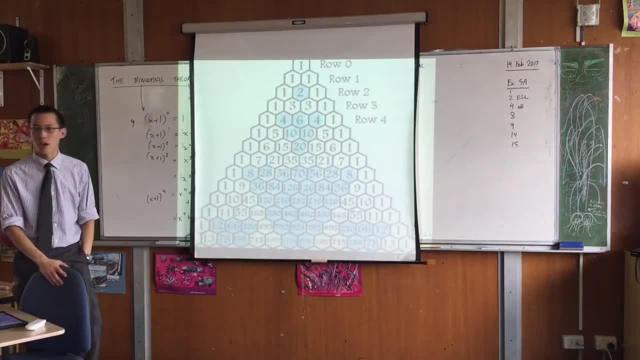 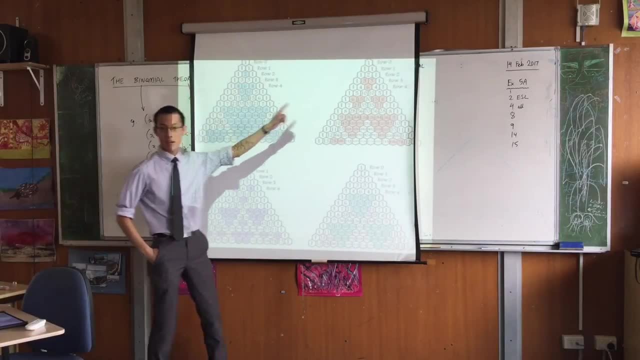 Think about where. Have a look at it again. Think about where the multiples of 3 are. Can you see some multiples of 3?? Do you see them there? There are the multiples of 3.. There are the multiples of 4.. 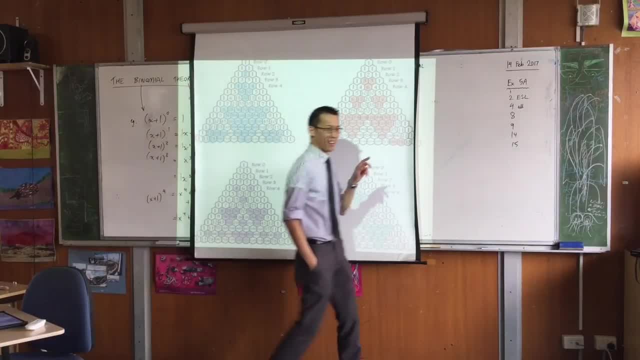 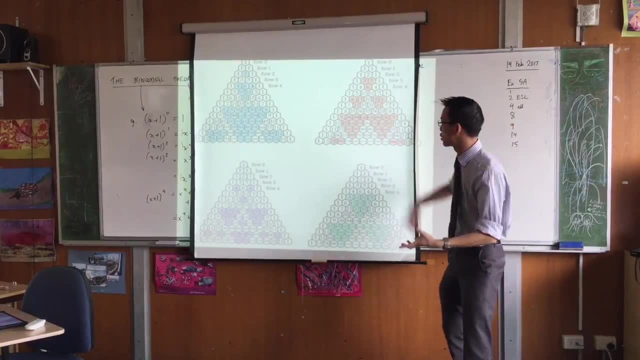 There are the multiples of 5.. I don't like to say this very much, but if there's any Blackfordian magic in mathematics, this has to be it, Because can anyone tell me to make all these numbers? where do they come from? They don't come from polynomials. Where do they come from, Like, for example, 1,, 2, 1.. Where do you just magic those numbers from There? The square of 11.. 121 is the square of 11.. 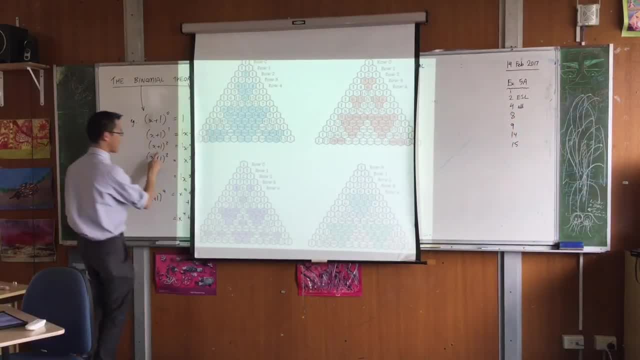 However, interestingly, that comes from this. It actually comes from this, Because the square of 11 is, of course, 10 plus 1.. Can you hear that? Yes, So it's really 10 squared plus 2 times 10 plus 1.. 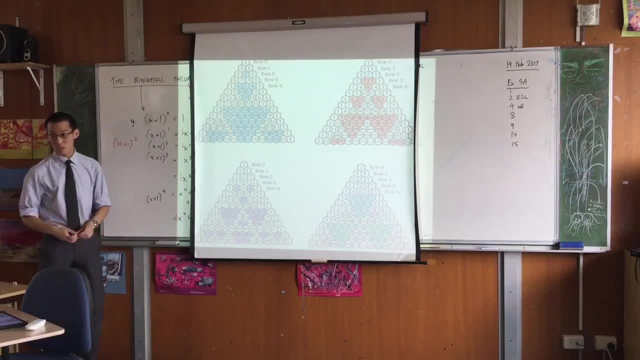 That's the 1,, 2, 1 that you're noticing, But there's actually a much simpler rule for people who can't square 11, because it's big numbers. You may have encountered this a long time ago To get 1,, 2, and 1,. 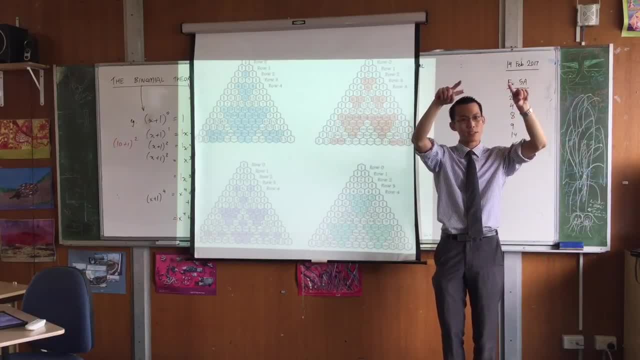 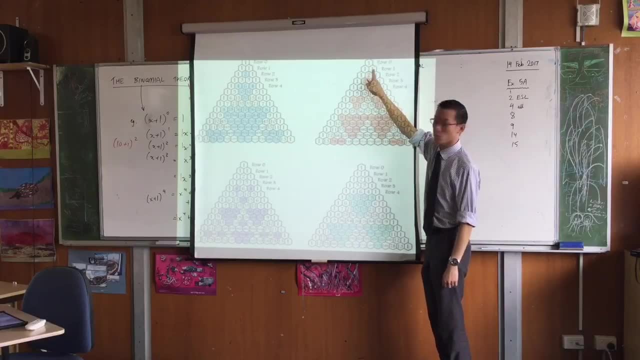 you just add together the numbers that are on the previous row. Do you recognise that? So this 2, you've got 1s going down the sides all the time, but the 2 comes from 1 plus 1.. Pick another random number. 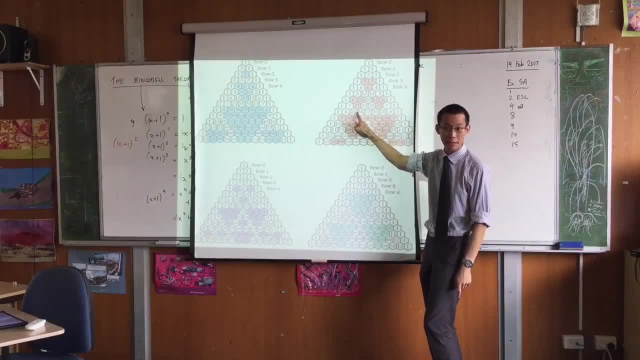 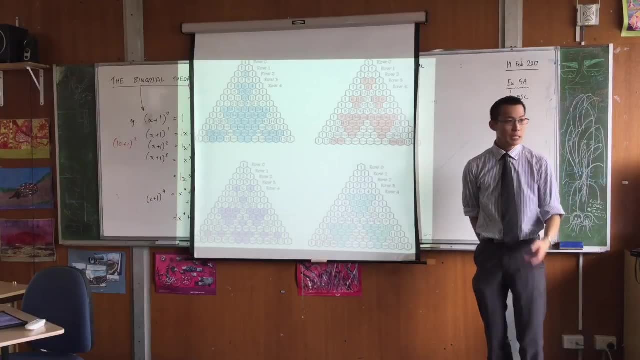 This 36,, for instance, That comes from 8 plus 28.. So all you need to know to make Pascal's triangle- and you will be making Pascal's triangle in a second- is just adding numbers, Just adding numbers. That's all that constructs this. 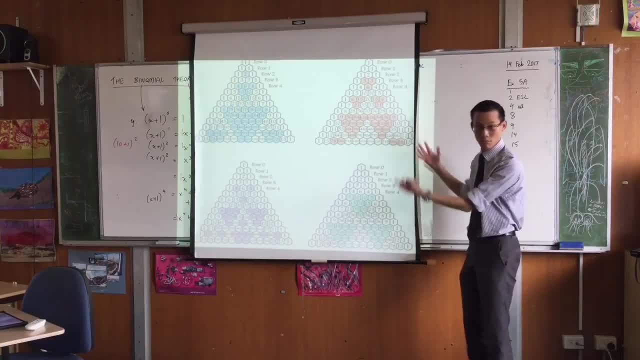 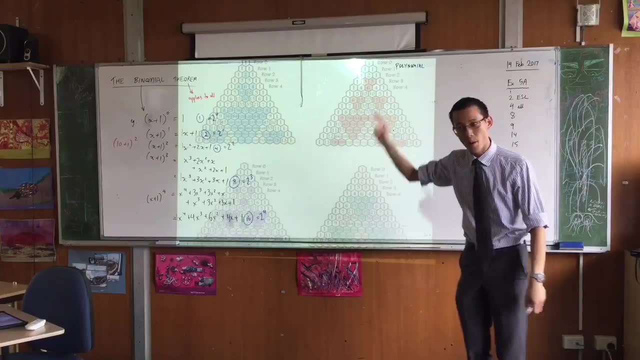 And yet somehow, number 1, you've got these weirdo-looking patterns. Number 2, what on earth does this have to do with anything? This is polynomials, binomials and how they expand. Why should this have anything to do with these? 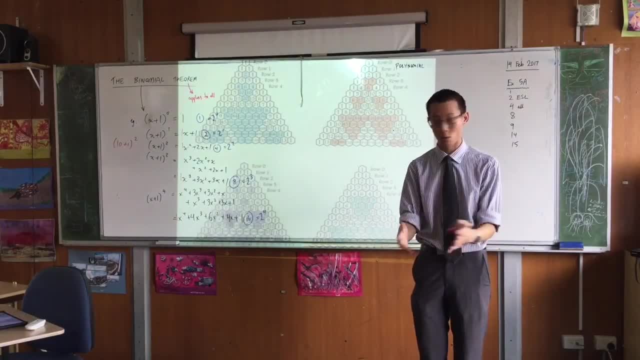 And that is a core mystery in this course that we will solve, but not quite yet.